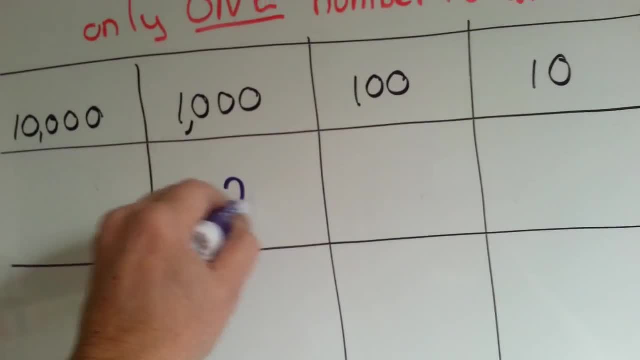 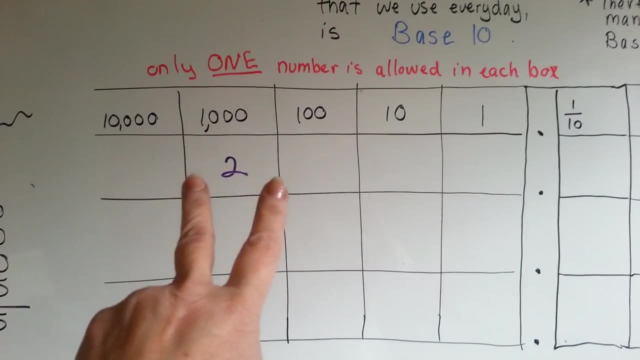 That means in the thousands place we have a 2. Now there's only one number allowed in each box, Because if you got to two numbers, like a 12, then in the 12, the 1 of the 12 should be in this box. 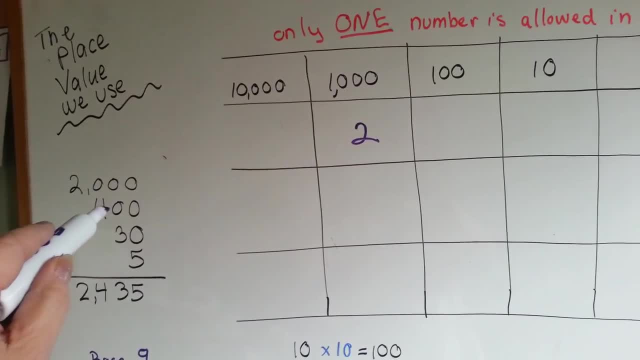 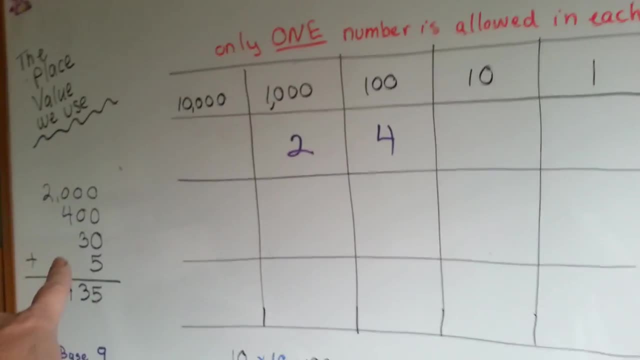 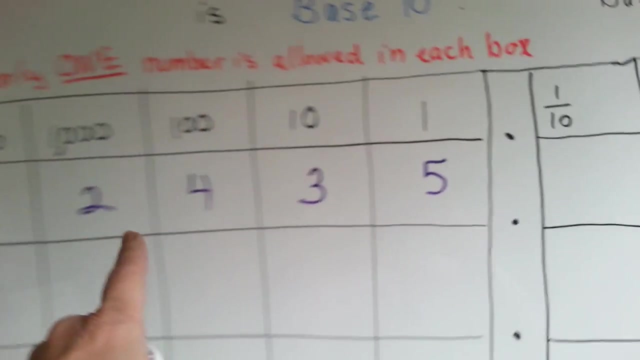 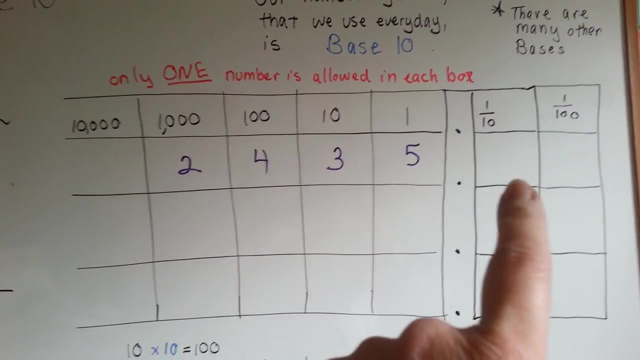 So 400 goes in the hundreds- We have four 100s. 30 means we have three 10s, And the 5 means we have five 1s. That is our base 10 system. One number goes in each box and it represents that group. 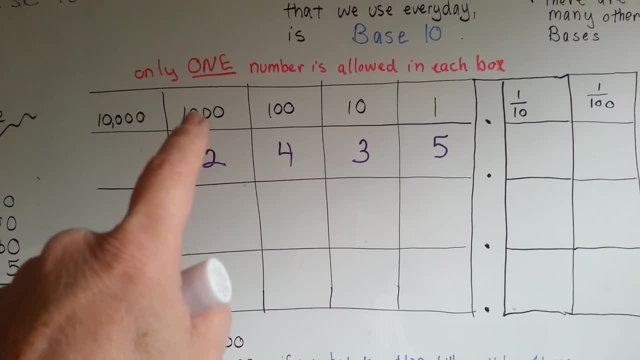 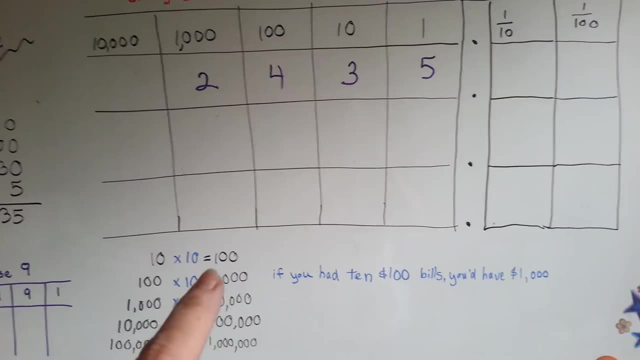 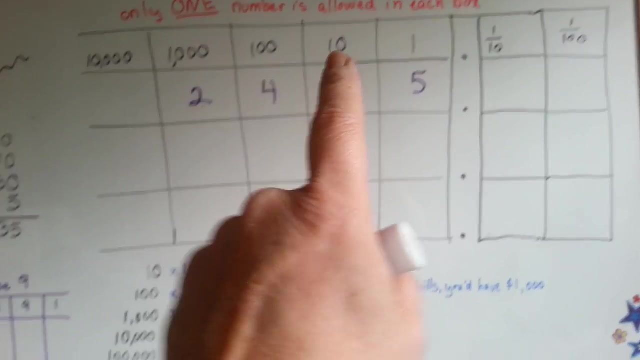 Two means two thousands, So that when we add them up, we get 2435.. Now look at this: 10 times 10 is 100.. So we went from 1 to 10.. 1 times 10 is 10.. 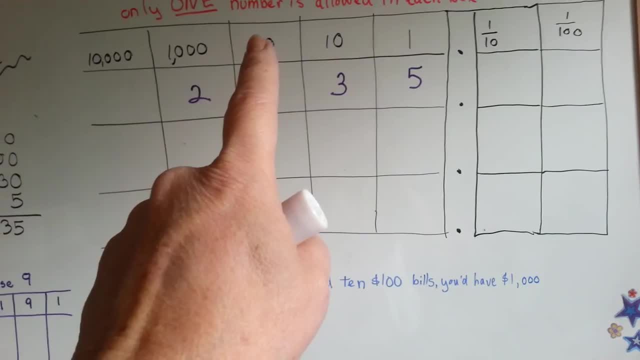 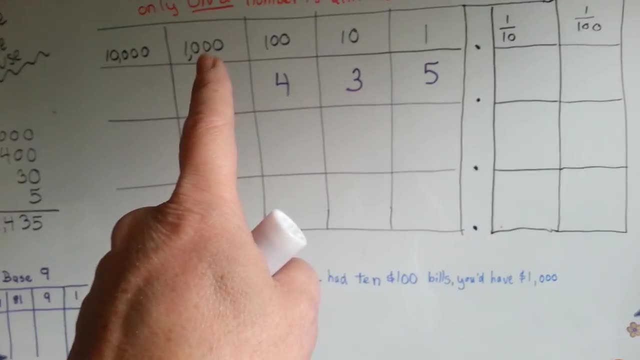 And now we're going to say: 10 times 10 is 100. And we're going to keep multiplying by 10 to get the next column. So 100 times 10 is 1000. If you had 10 $100 bills, you'd have $1000. 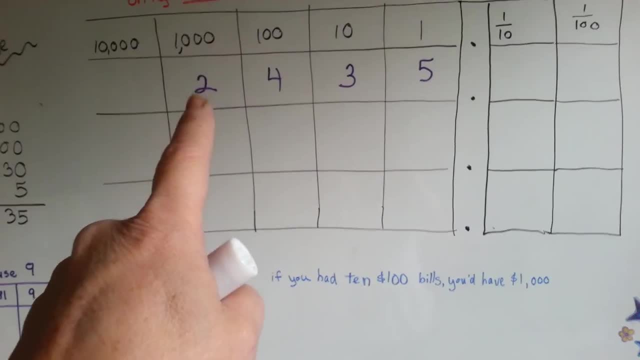 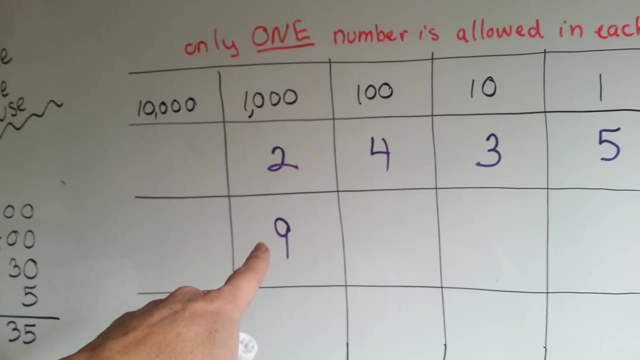 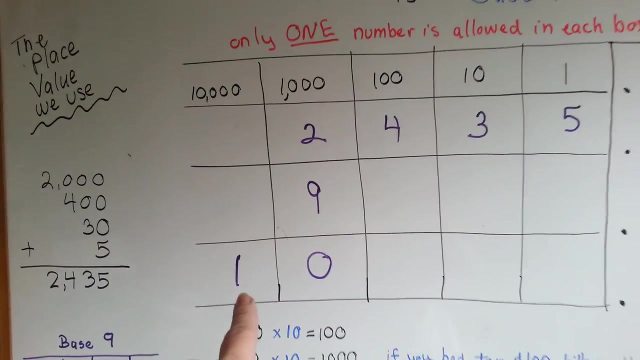 Okay, So once this here got to 9,. that's as high up as you can go. It can't go to 10.. Because if you did, then it would look like this: Because only one number is allowed in each box. 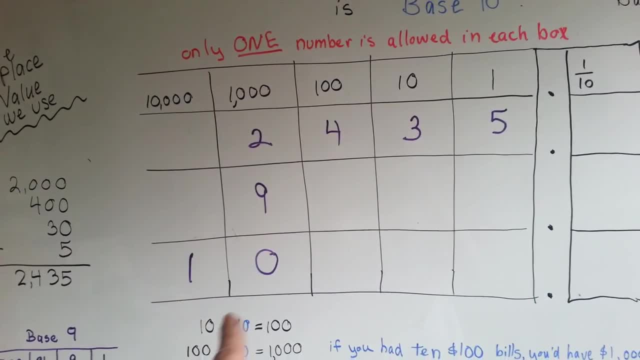 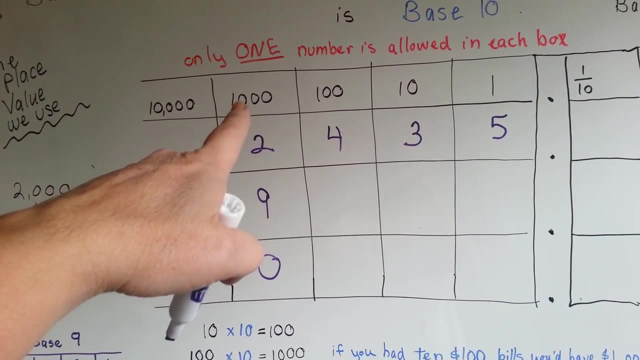 That means you'd have one 10,000 and zero thousands. You'd have 10,000. See, It goes from 9,000 to 10,000. So the one that one 10,000, would be in that box. 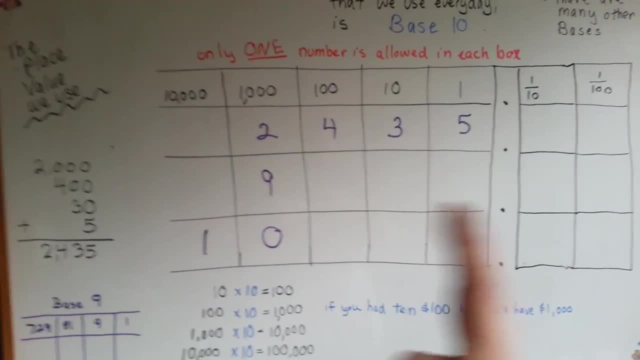 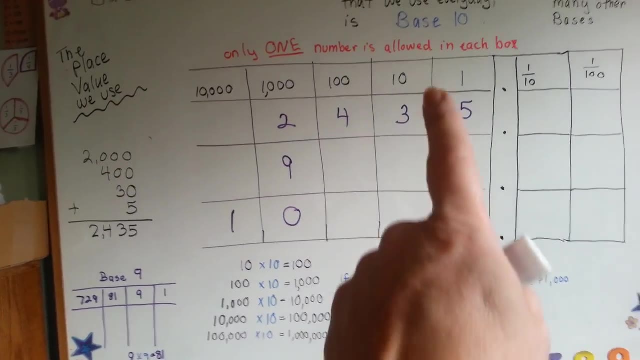 That's the way our base 10 system works. One number in each box, You multiply it by 10.. 10,000 times 10 is 100,000.. 100,000 times 10 is a million, And that's how you know what goes up here. 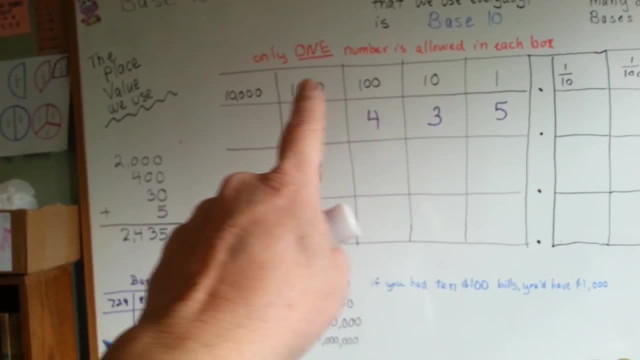 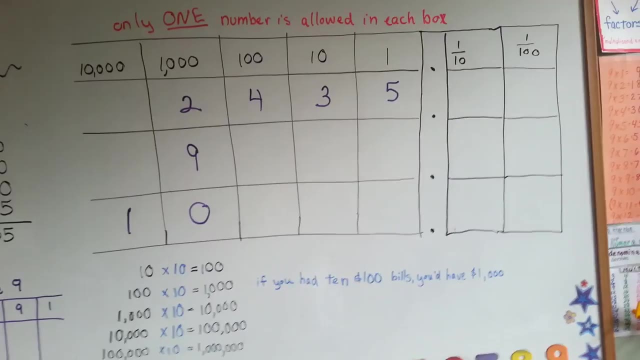 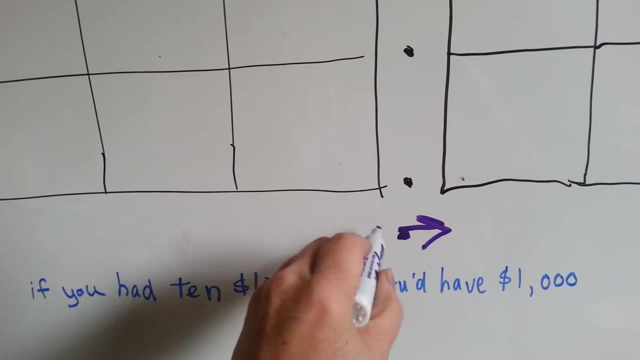 In this row up here is that each one is multiplied by 10, heading off to the left, Going this way, on this side of the decimal point, from this point, this way, you're this side here. let me do this. 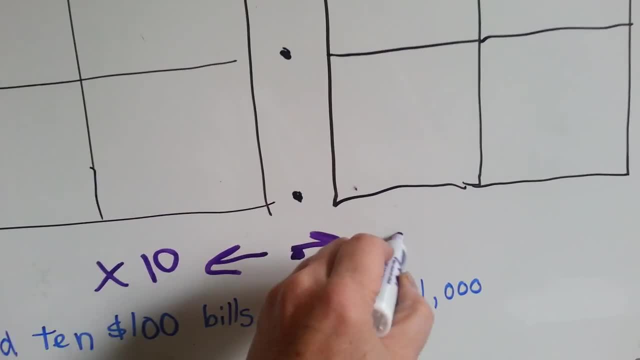 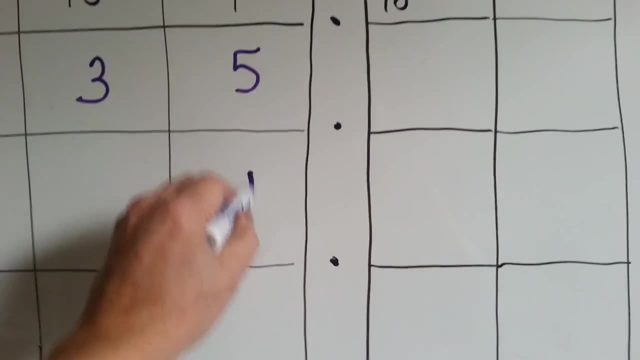 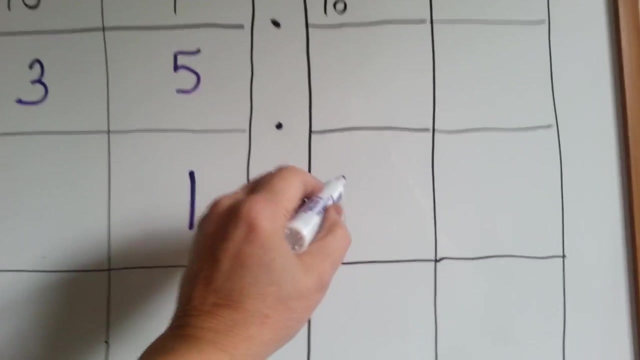 On this side, you're multiplying by 10.. When you go this way, you're dividing by 10.. Okay, So if you have a 1, in the ones column and you want to go this way, you're splitting that 1 into 10 parts. 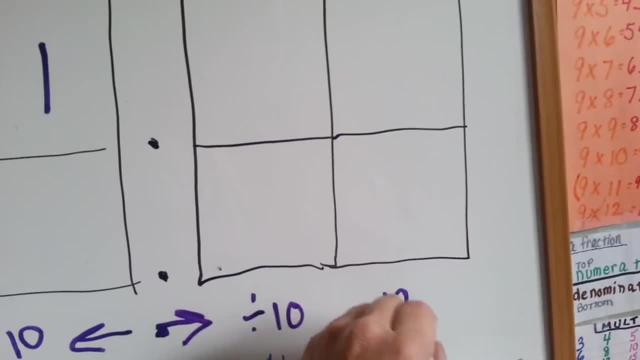 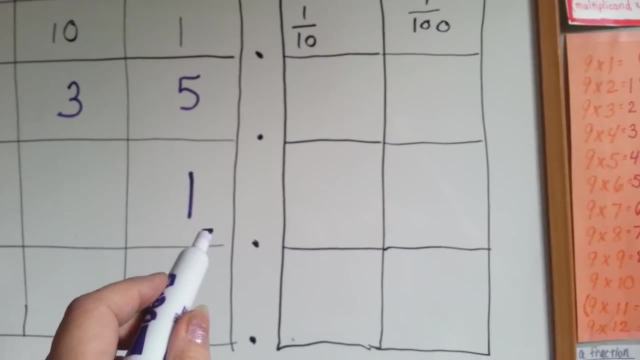 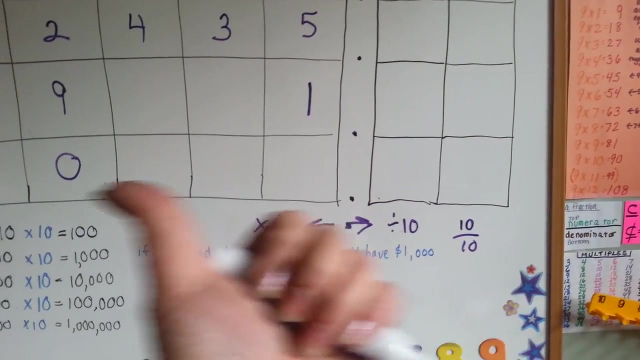 It's like saying you have 10 tenths. 10 tenths is 1.. Okay, You would have to divide it by 100 to get into this column, See. So this is dividing by 10.. This side is multiplying by 10.. 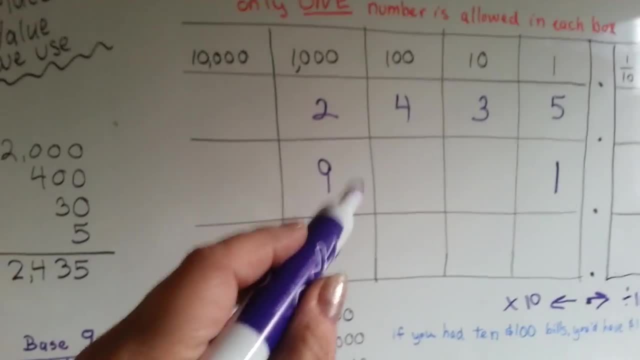 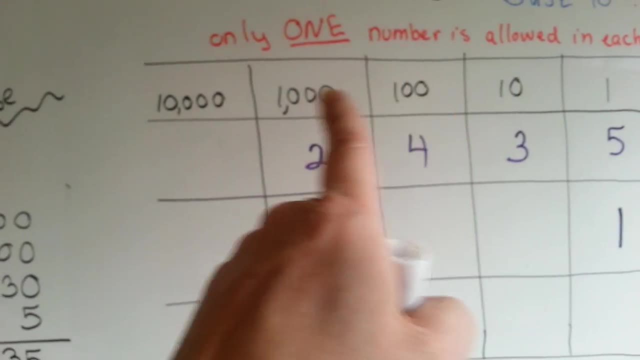 Now let's look at this base 9, so that you can understand the difference between base 10 and another base. In base 10, we say ones, tens, hundreds, thousands. In base 9, we say one, nine, eighty-one. 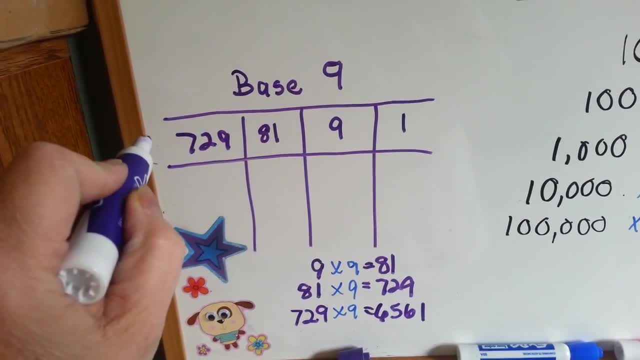 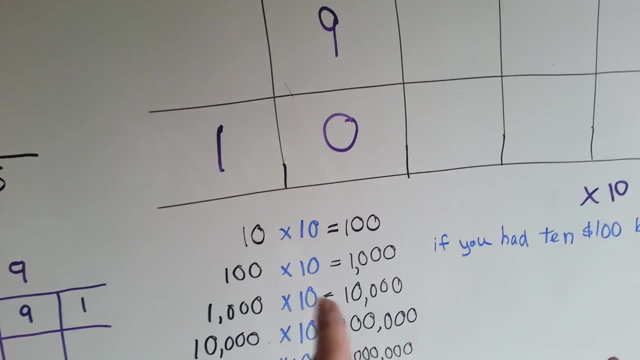 seven hundred and twenty-nine, And the next number over to the left would be 6,561.. Now, why is that? Well, because in the base 10, we were multiplying by 10 to get to our next number to the left. 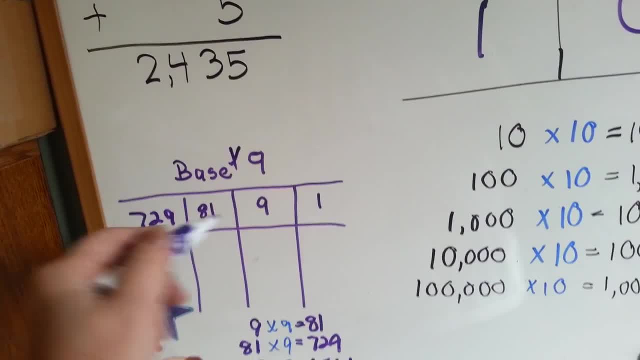 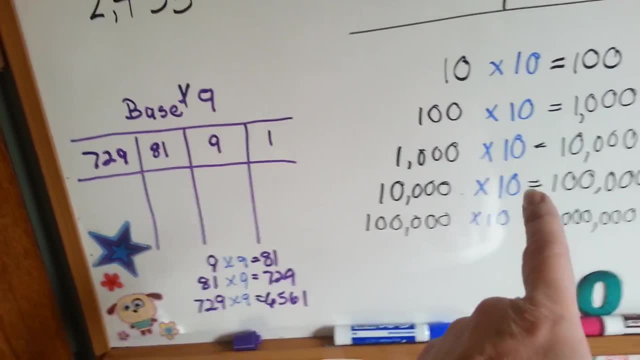 In base 9, we multiply by 9 to get to the left. So 1 times 9 is 9.. So that's our 9.. 9 times 9 is 81. See Over here we were saying: multiply by 9.. 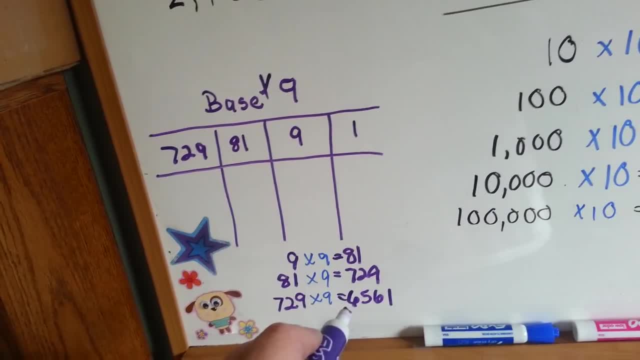 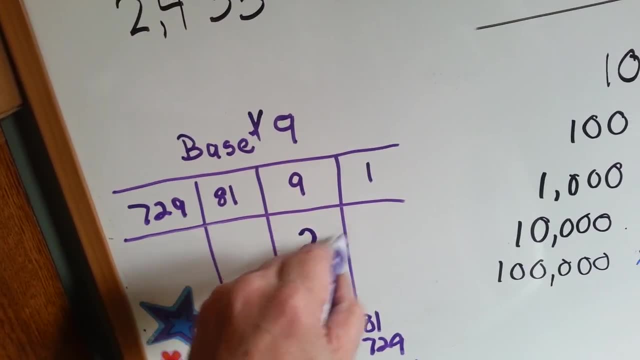 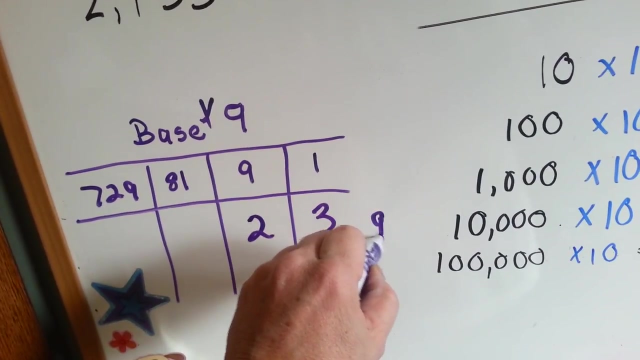 81 times 9 is 729.. 729 times 9 is 6,561.. So in base 9, this number means two 9s and three 1s, Two 9s and three 1s, And if you were to add that up, 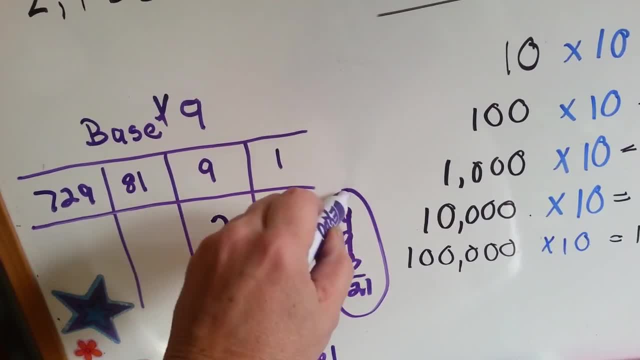 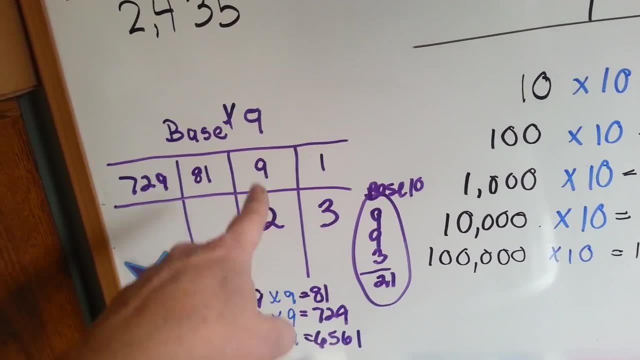 you'd have 18,, 19,, 20,, 21. But that would be in base 10.. In base 10, it would be 21.. But in base 9, it's 23, because that means there's two 9s and three 1s. 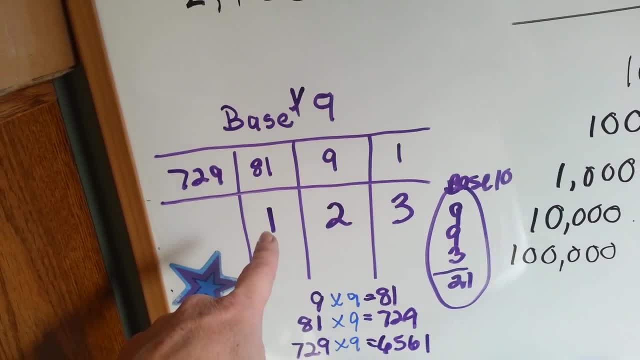 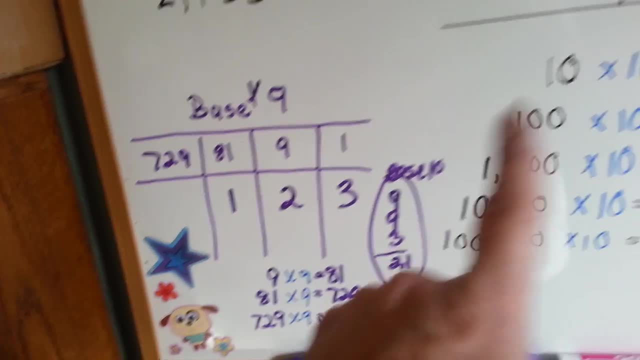 If we said that there was one here, that means there's an 81,, two 9s and three 1s. See how base 9 is different than base 10? So in my next video I'm going to go over base 9 again. 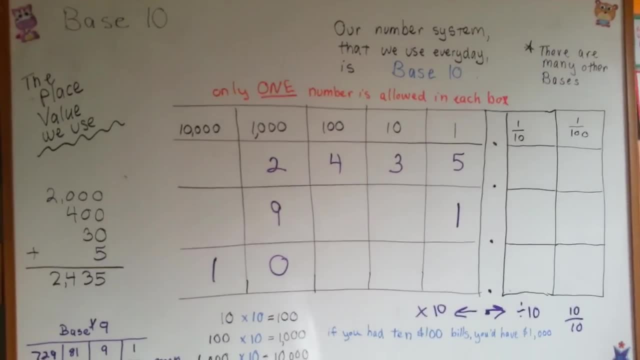 and I'm going to explain it, And I will go all the way to base 2, which is binary. So stick with me. This is kind of fun. It's like a puzzle. 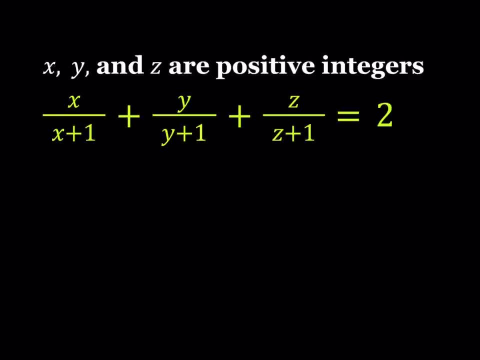 Hello everyone, In this video we're going to be solving a Diophantin equation. x, y and z are positive integers and we have this equation. So one of the things we're going to do to solve this problem is we're going to first of all separate this into pieces. 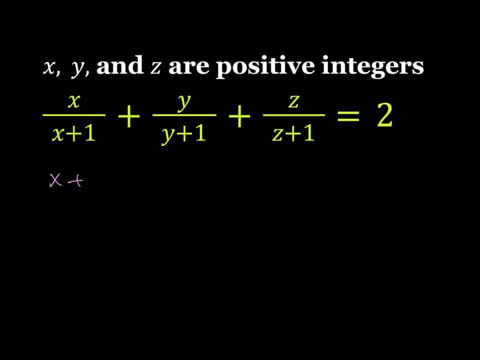 So I'd like to write x as x plus 1 minus 1 divided by x plus 1.. Now this is going to allow me to separate the 1 and write it as 1 over something. So I'm going to be doing this for everything here. 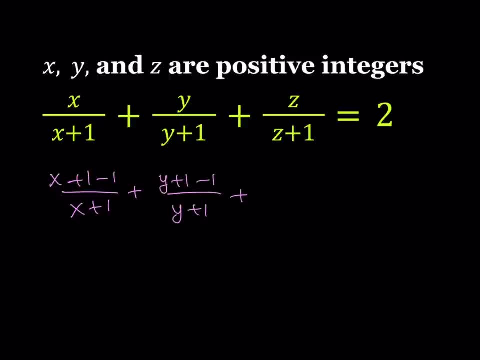 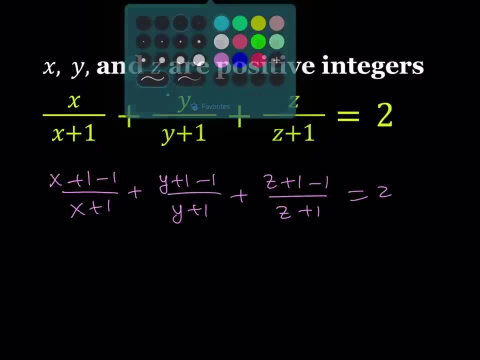 y plus 1 minus 1 and z plus 1 minus 1.. So, from here, notice that we're going to be getting x plus 1 over x plus 1, which is 1,, another 1, and another 1.. 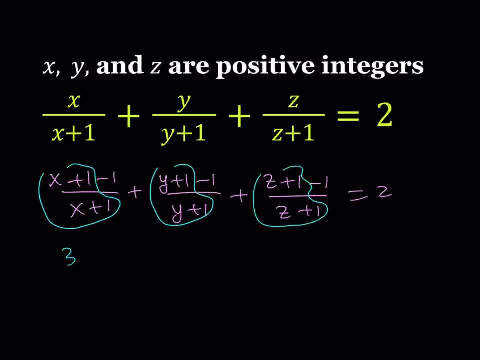 So the sum of these 1's is going to be 3.. So we're getting 3 minus 1 over x plus 1, minus 1 over y plus 1, minus 1 over z plus 1, and the whole thing is equal to 2.. 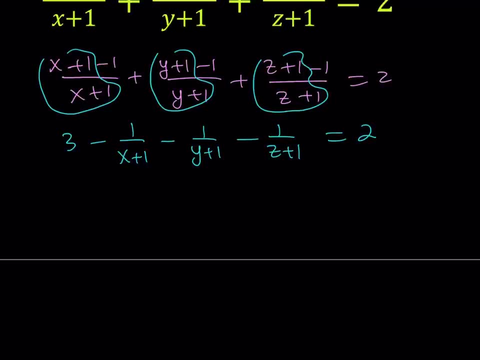 Now we can just go ahead and take everything on the left hand side except for the 3 and put it on the right hand side by adding: and we should be getting 1 over x plus 1 plus 1 over y, plus 1 plus 1 over z plus 1 equals 3 minus 2, which is 1.. 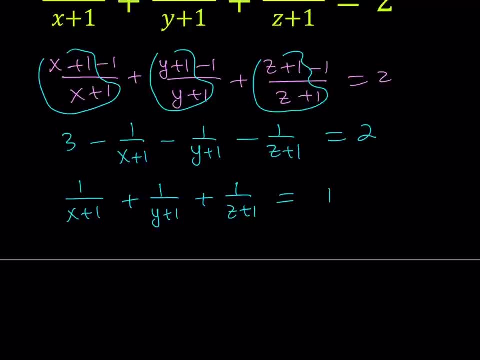 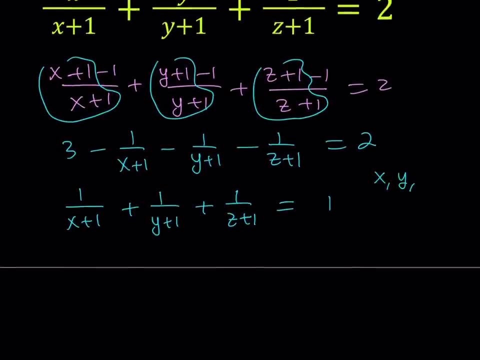 Okay, So now we have the sum of 3 reciprocals and it equals 1.. Now, if you remember, x, y, z have to be positive integers. So x, y, z are all greater than 0, right? Or we can say greater than or equal to 1.. 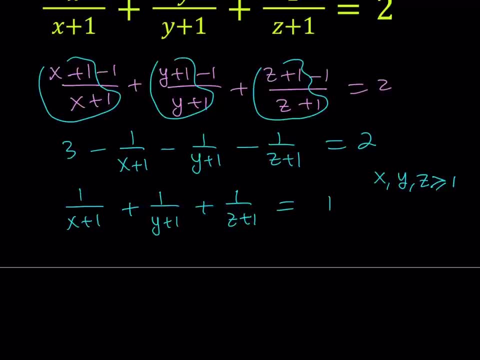 But now we do have a different situation. here We have the x plus 1. So let's go ahead and use substitution. As you know, substitution is one of my favorite methods. Let's call this a, let's call this b and let's call this c.